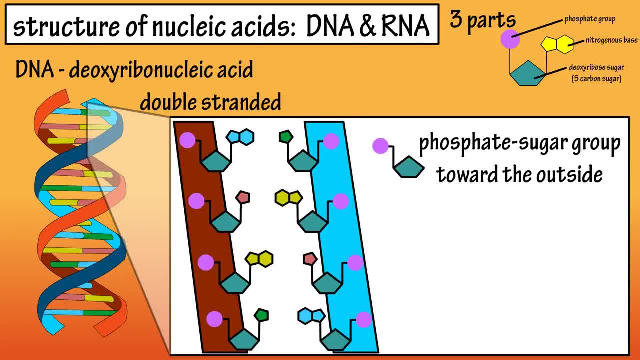 helical chain has its phosphate sugar group toward the outside and the nitrogenous bases facing inwards towards the nitrogenous bases of the other chain. Each of the bases on one chain is joined to the base of the other chain through either two or three hydrogen bonds. 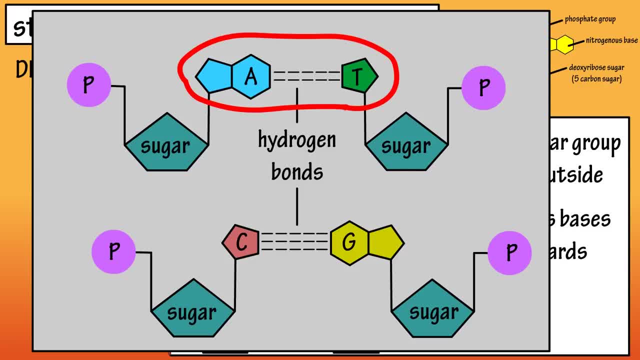 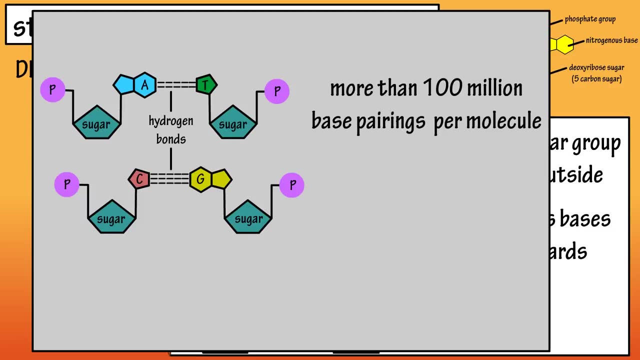 Thymine and adenine are joined by two hydrogen bonds, and cytosine and guanine are joined by three hydrogen bonds. Thymine and adenine are always a base pair, and cytosine and guanine are always a base pair. It's estimated that DNA molecules contain more than 100 million of these. 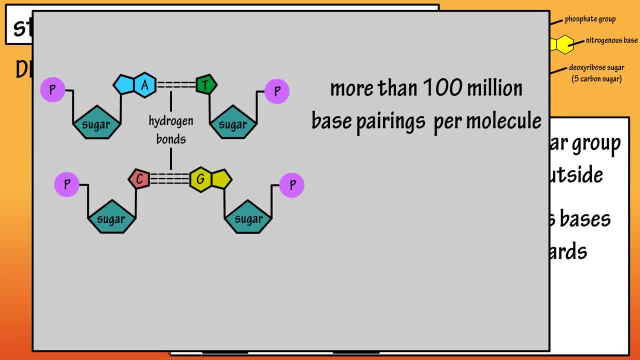 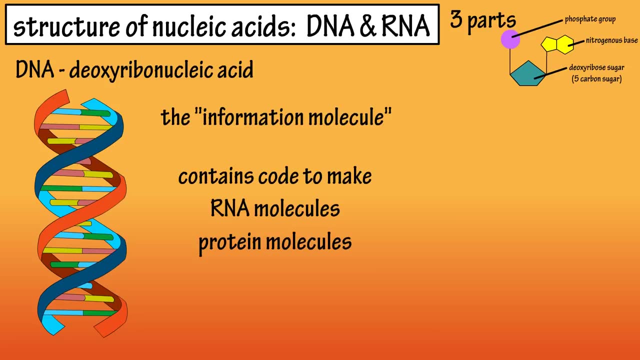 base pairings and in one individual's body. the sequence of the base pairings is the same in every DNA molecule, So this sequence of base pairing is unique to that individual. DNA is often called the information molecule because it contains the master code needed to make various RNA molecules. 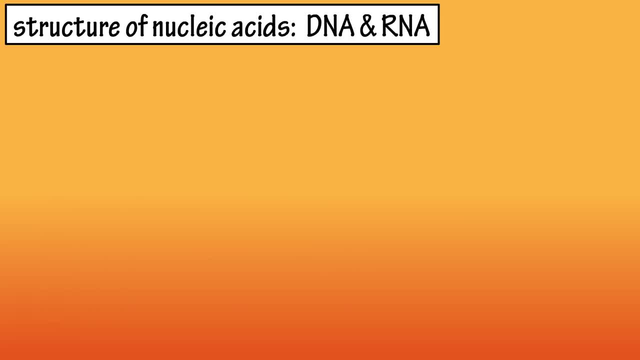 and protein molecules in the body. Now for RNA. The nucleotides that make up RNA are very similar to those that make up DNA. RNA nucleotides have a phosphate group with the same structure as in DNA. They have a five carbon sugar, but the number two is a five carbon sugar. 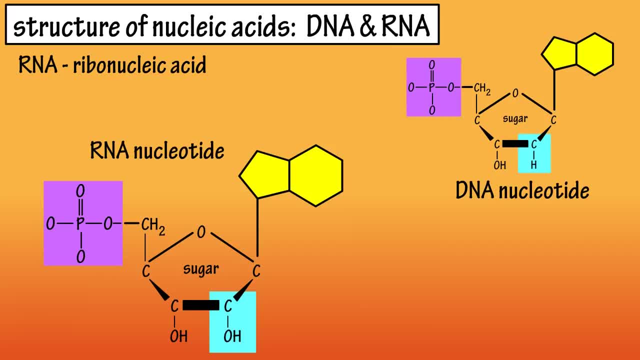 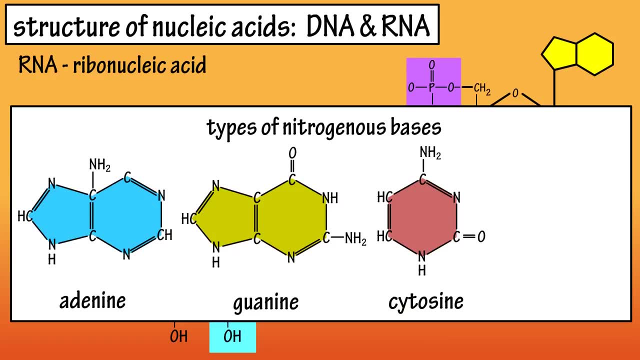 Carbon is bonded to a hydroxyl OH group instead of a lone hydrogen atom, and this sugar is called ribose. It also consists of the three same nitrogenous bases as DNA, cytosine, adenine and guanine, but it does not contain thymine. Instead, it contains uracil, which is a single 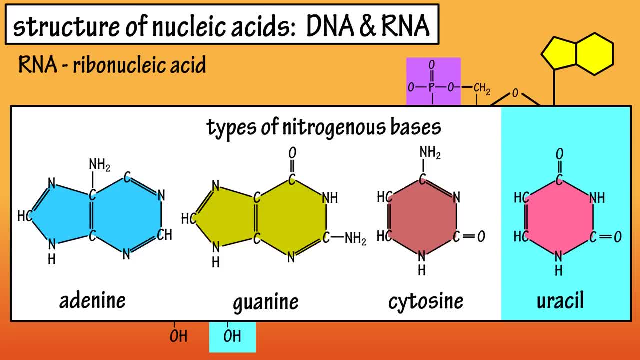 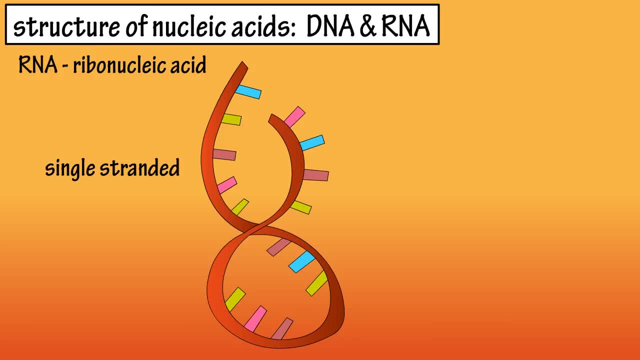 ring structure like thymine, making it a pyrimidine base. Most RNA molecules are single-stranded nucleic acids and many times they form a folded, compacted structure with some hydrogen bonding taking place within the base pairs of the molecule. These pairings are the same as in DNA. Cytosine and guanine are a base pair. 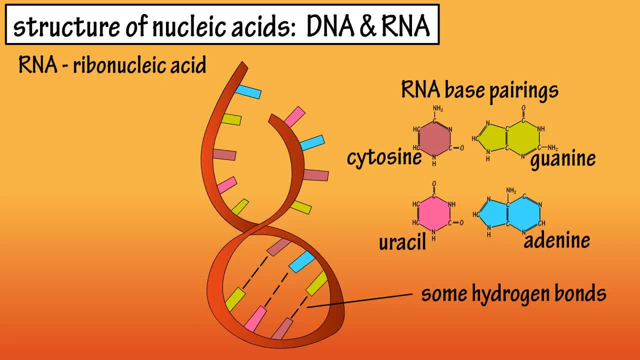 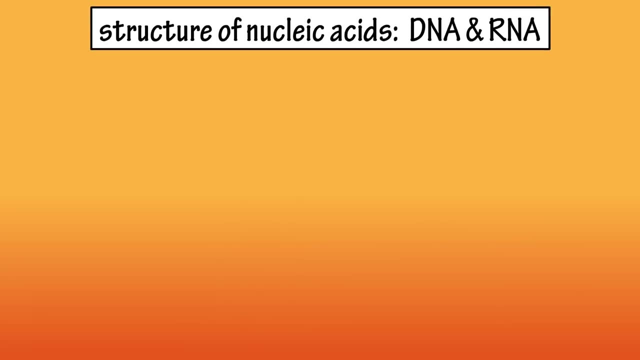 and uracil takes the place of thymine and pairs with adenine. RNA is extremely important in the process of forming different proteins in the body, of which we will cover in depth in a later video. And that be the basics on the structure of DNA and RNA. Thank you for watching.